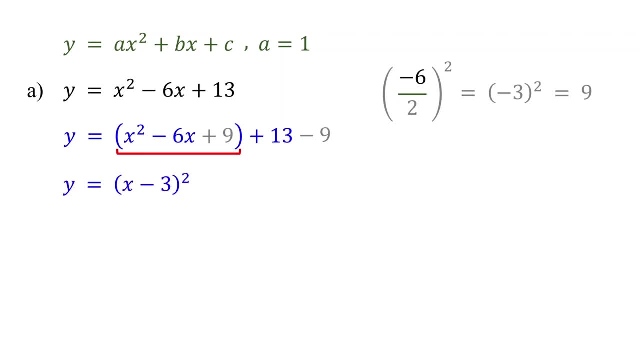 trinomial as a binomial square, which will be x minus 3 squared, The number in the binomial always corresponds to half of the coefficient of the x term in the perfect square trinomial, which in this case is negative, 3.. 13 minus 9 equals 4.. 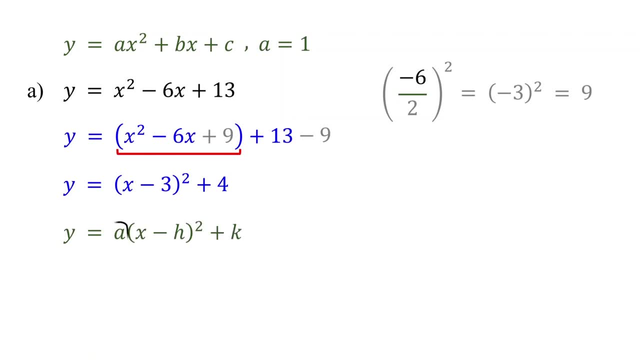 This is now in vertex form, where a equals 1.. h is the opposite of the number inside the parentheses. This is now in vertex form where a equals 1.. h is the opposite of the number inside the parentheses And k equals the constant term. From this we can tell that the vertex is the point 3 comma 4.. 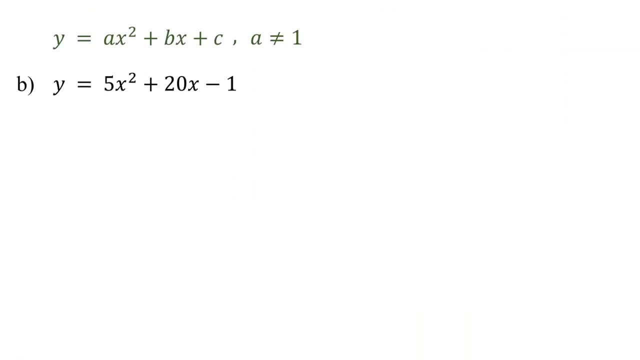 And k equals the constant term. From this we can tell that the vertex is the point 3, comma 4.. In the next example, the leading coefficient is different from 1.. What should we do first in this case? Remember to complete the square. the leading coefficient. 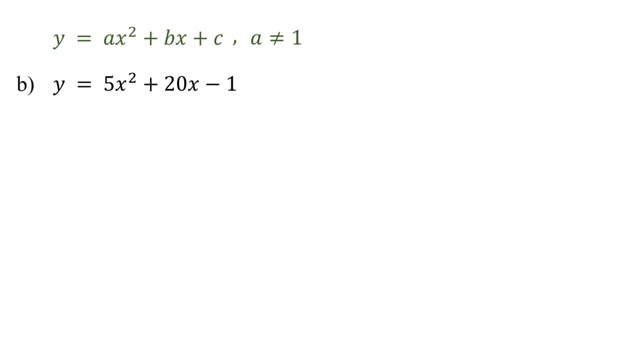 must be 1.. So when the leading coefficient is different from 1,, our initial step is to make it 1.. We do this by factoring it out from the variable terms. Here the leading coefficient is 5.. Factoring it out from the variable terms gives us 5 times x squared plus 4x. 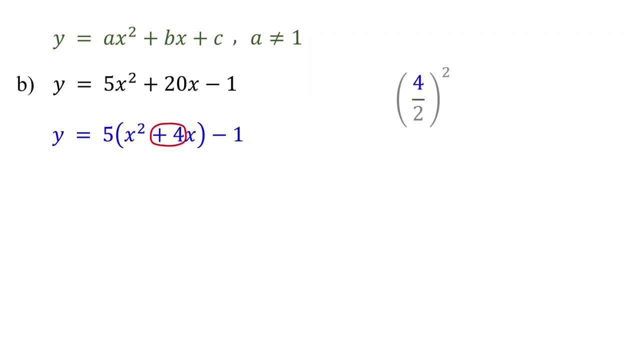 Next, find half of the coefficient of the x term and square it. Half of 4 is 2, and 2 squared equals 4.. Then add this value to the variable terms inside the parentheses to complete the square. This is now a perfect square trinomial. Now to maintain the equation value: 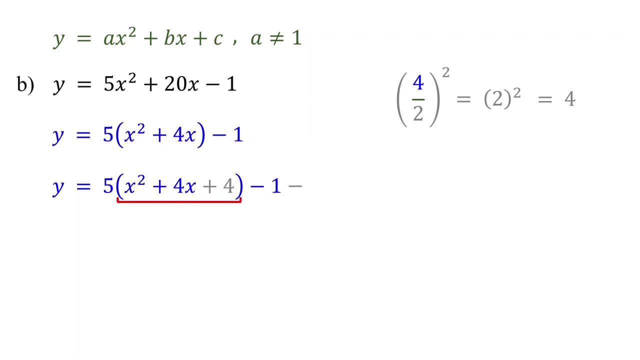 what number should we subtract? What do you think? Notice that the trinomial is multiplied by 5.. If we distribute 5, 5 times 4 gives us 20, which means we are actually adding 20, right? So to maintain the equation value, we must subtract 20.. 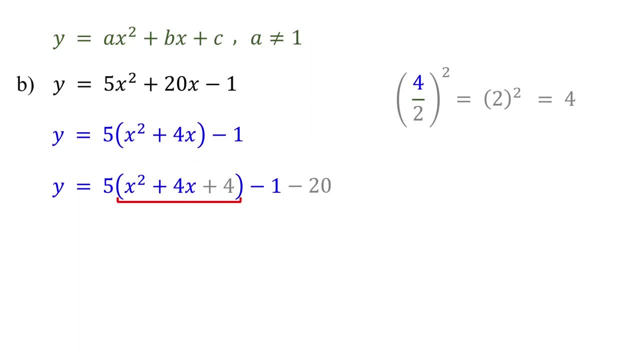 Next rewrite the perfect square trinomial as a binomial square, which will be x plus 2 squared. The number in the binomial is half of the coefficient of the x term. in the perfect square trinomial, Negative 1 minus 20 equals negative 21.. This is now in vertex form. 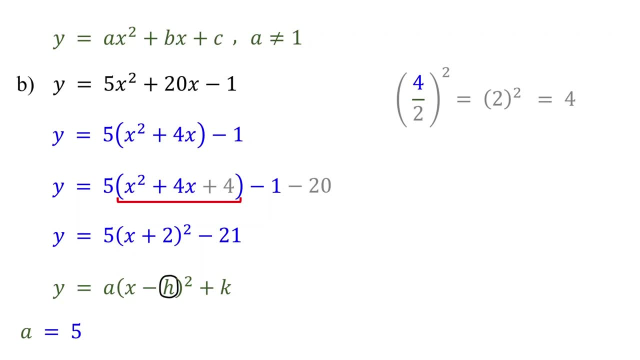 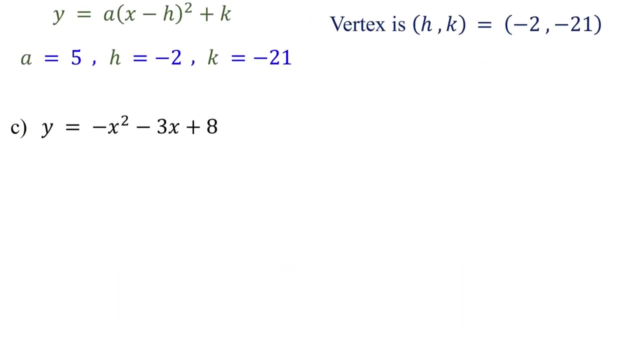 where a equals 5, h equals the opposite of the number inside the parentheses and k equals the constant term. So the vertex is the point: negative 2 comma, negative 21.. Let's work on one more example with a leading coefficient different from one, and also a bit. 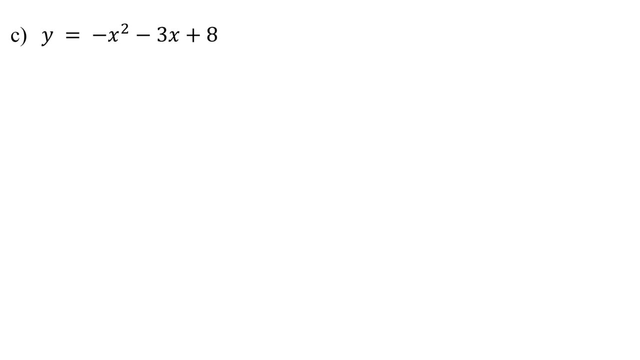 challenging. Feel free to pause the video and give it a try. The leading coefficient is negative 1, so our initial step is to factor it out from the variable terms. This gives us the negative of x squared plus 3x. Next, find half of the coefficient of the x term and square it. 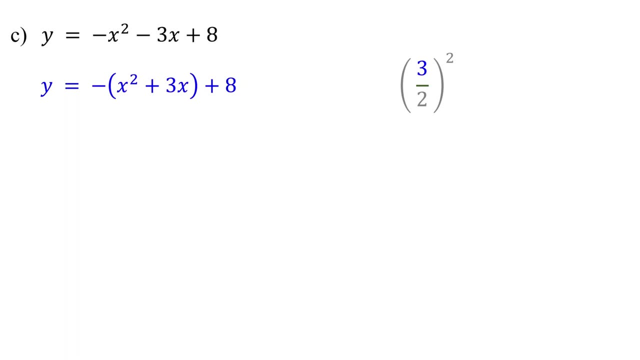 Since 3 does not divide evenly by 2, we leave it as a fraction: 3 squared is 9, and 2 squared is 4.. Then add this value to the variable terms inside the parentheses to complete the square. This is now a perfect square trinomial. 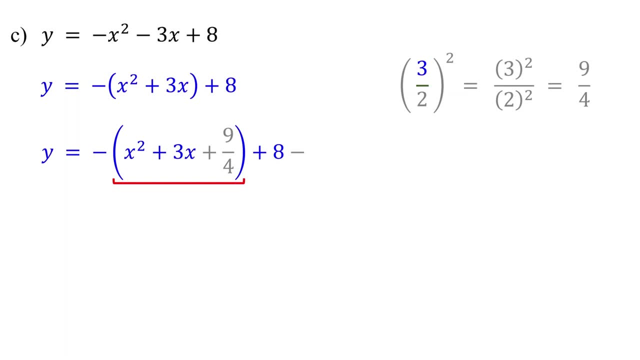 Now to maintain the equation value, what number should we subtract? Notice that the trinomial is multiplied by negative 1.. If we distribute negative 1, negative 1 times 9 fourths gives us negative 9 fourths, which means we are actually adding. 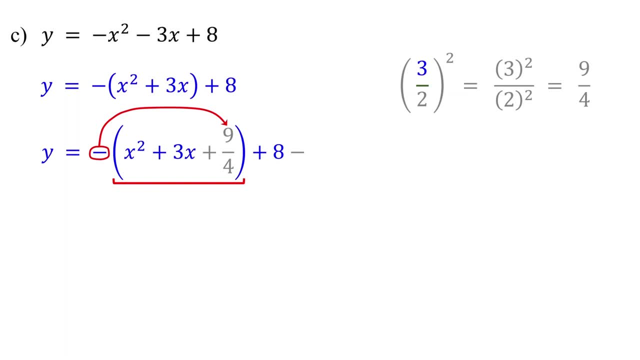 negative 9 fourths Right. So to maintain the equation value, we'll also make a NOTHING plus X to the root of the cube. We then multiply by one. So we have negative 1 minus 3 square squared. and now let's completely Sanders. 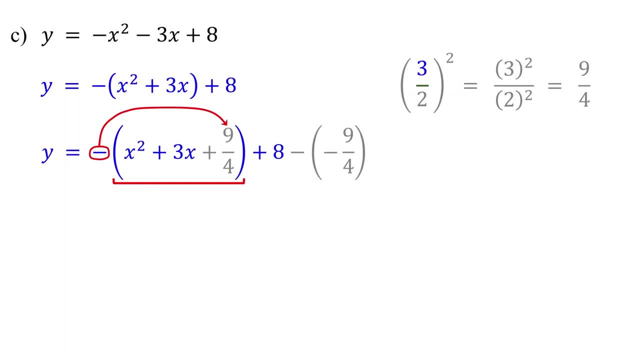 To maintain the equation value, we must subtract negative nine-fourths. Next, rewrite the perfect square trinomial as a binomial square, which will be x plus three-halves squared. The number in the binomial is half of the coefficient of the x term in the perfect square trinomial. 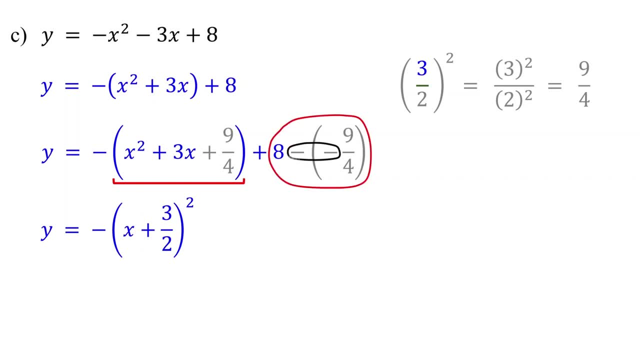 Now let's simplify this, Since negative times negative is positive. this is the same thing as eight plus nine-fourths right Eight is equivalent to eight over one. To get a common denominator, multiply it by four over four. Eight times four is thirty-two, and one times four is four. 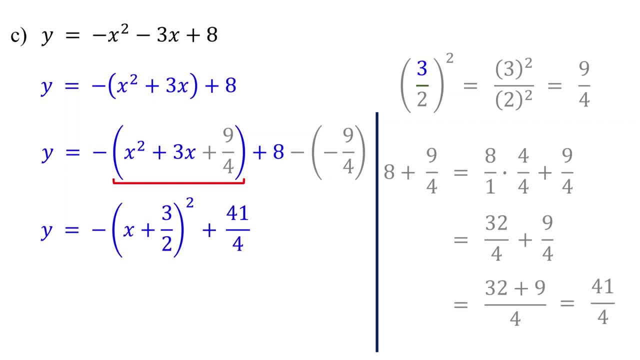 Now add the numerators, which equals forty-one. This is now in vertex form. A equals negative one, H equals the opposite of the number inside the parentheses And k equals the constant term. So The vertex is the point: negative three-halves comma. forty-one over four.